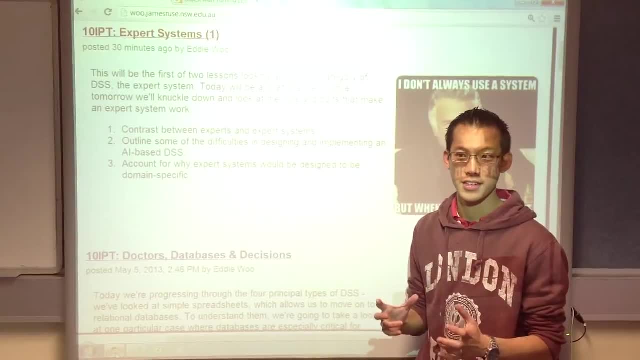 these points that I'm going to go through, because I've got quite a few. I'm going to mainly dwell on the advantages. I haven't found any pictures for the disadvantages. Maybe you can do me a favour and search up some of those. 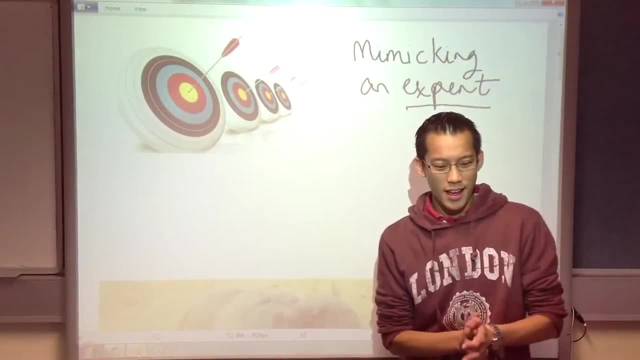 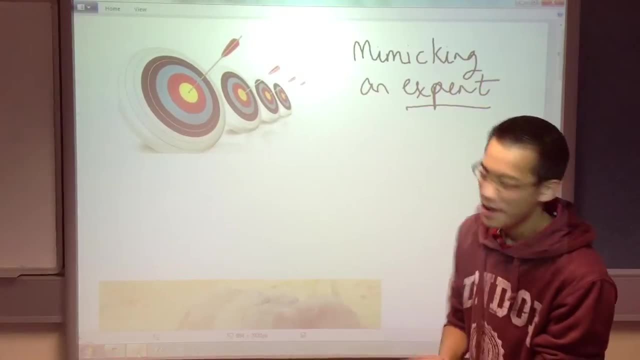 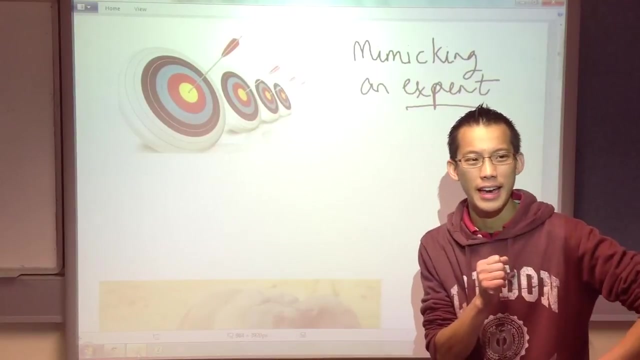 So let's go through these in order. Advantages first, of expert systems over their human counterparts. Number one: this is my picture, for accuracy is a tricky one. We'll deal with accuracy in a minute. I think you can argue that an expert system 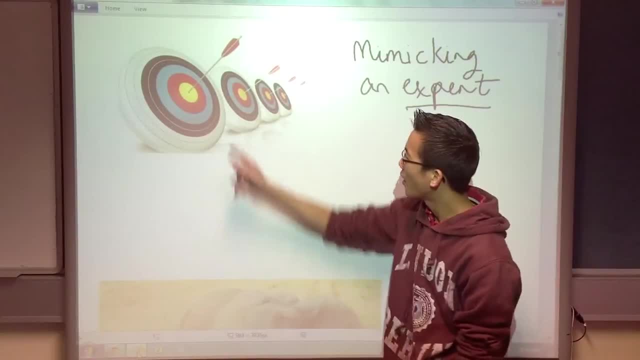 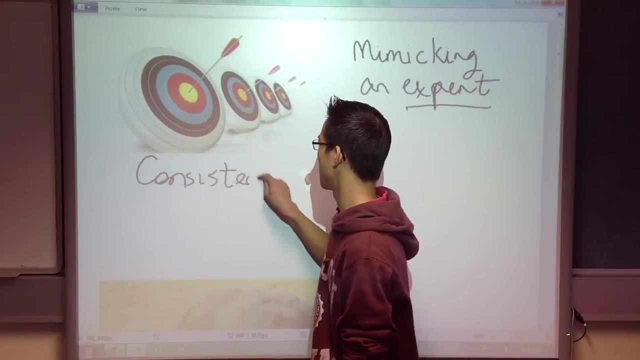 versus an expert might be more accurate, might be less. What I was really trying to get at with this- and maybe you can tell me if you can get a better picture- is about consistency. So here's the benefit of an expert system, a computer-based thing. 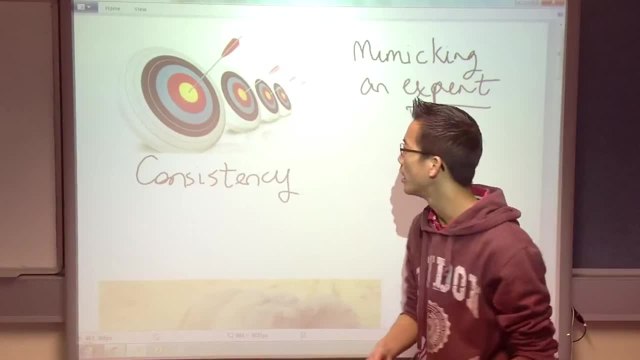 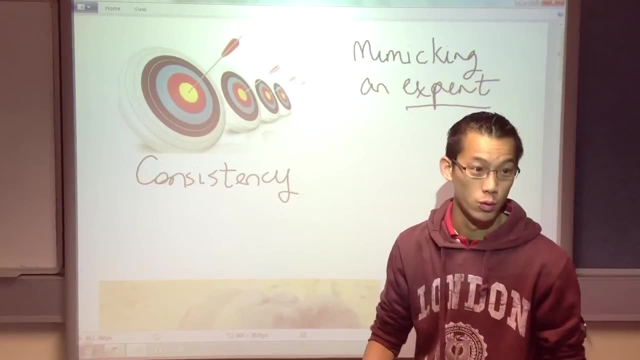 assuming it has all the logic and all the knowledge programmed into it. if it meets the same situation, this expert system- because it's a computer and all it's doing is following rules and logic- it's going to make the same decision again and again, and again. 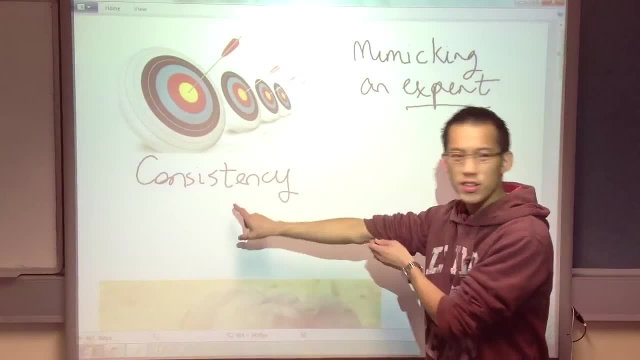 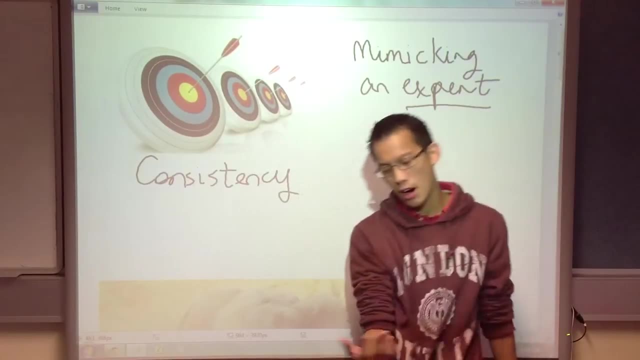 Now, later on we'll look at how that's a disadvantage, but can you see how that is an advantage? For instance, have you ever been frustrated when you get an exam back or something like that, and you're looking at it and you're like, oh, I lost marks for this? 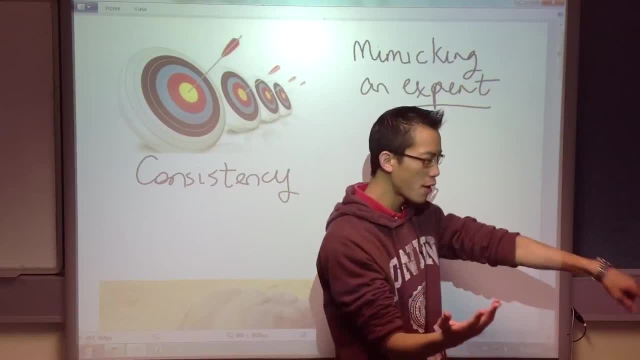 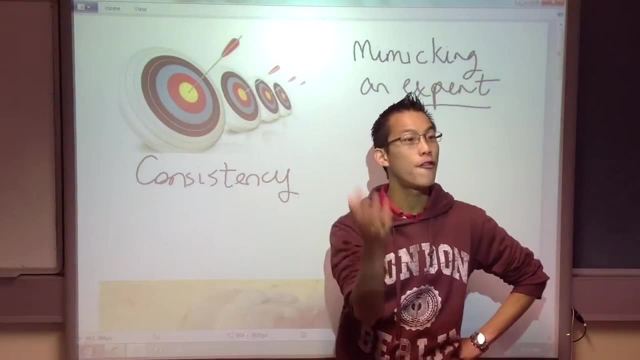 no big deal, This particular error. and then you look over at your friend and they made exactly the same error. their working looks identical, but they didn't lose any marks. What's wrong with that? That's not fair, is it? So consistency is about. 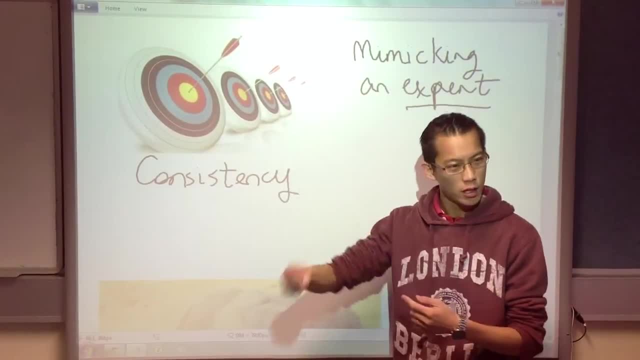 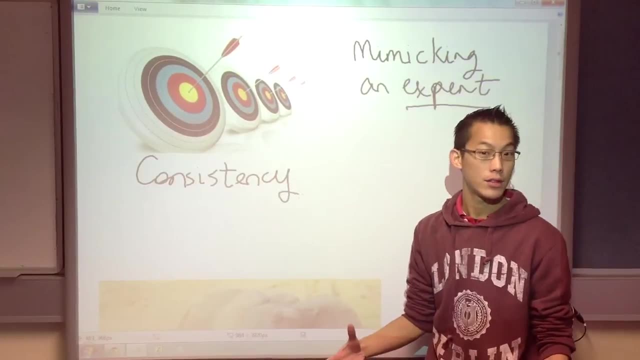 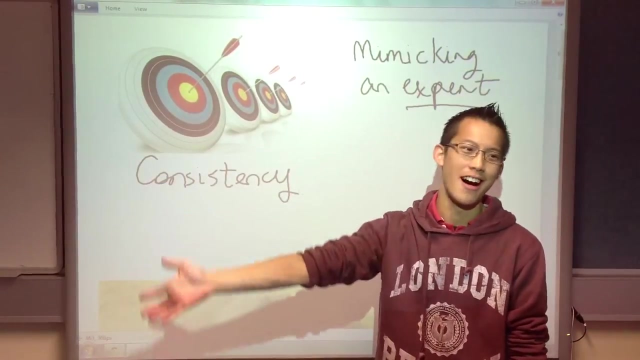 the computer's ability to always be following its understanding and its knowledge and its rules for how it makes decisions in always the same way in every situation. So that's a plus. Just human error, you know, we often say when a marker is tired or when someone is having a bad day. 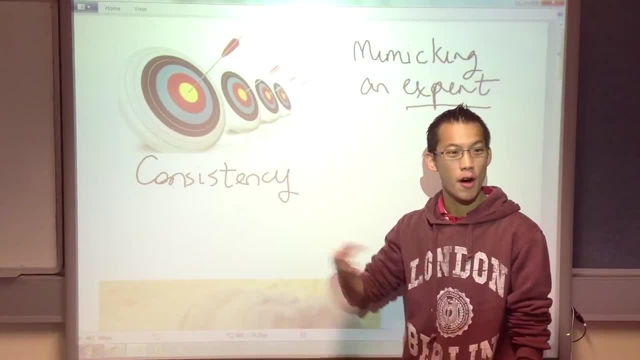 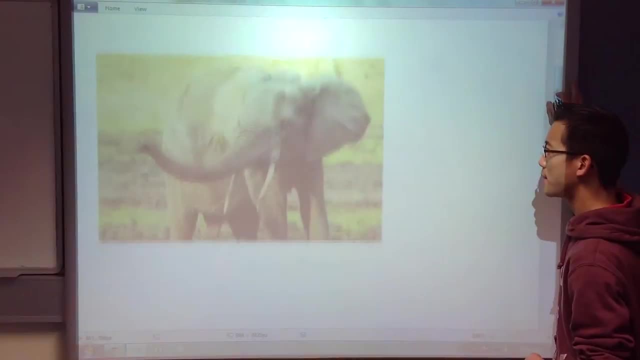 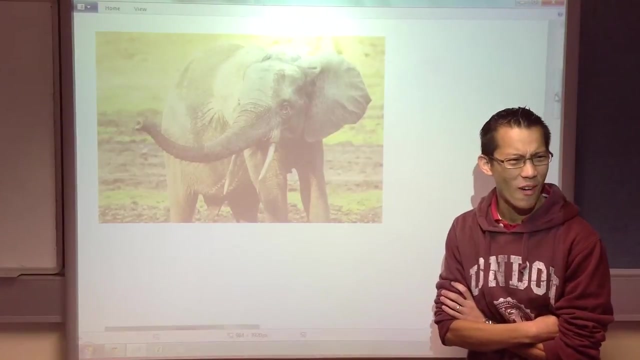 or something like that, then consistency can often go out the window. So humans and their subjectivity can be a problem. So, number one: consistency. Number two: any takers, Any takers. Morals, Elephants and morals. What are elephants? Elephants are famous. 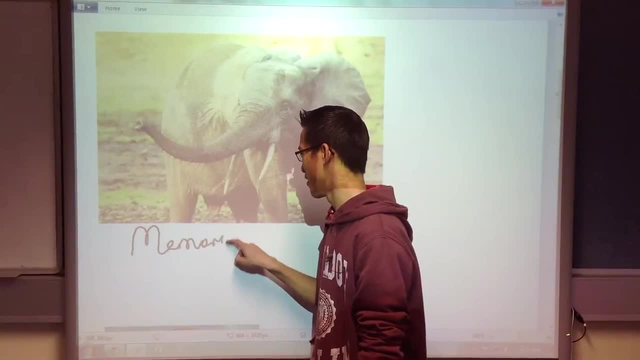 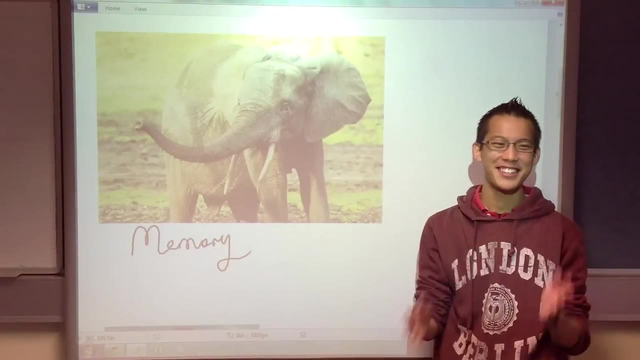 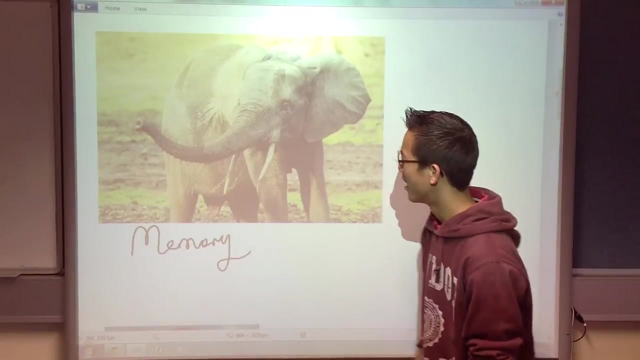 for memory. You've got memory over there Because we're killing elephants. That was the wow, nice work, Anyway. so what do I mean here? Well, they say: you know, wow, you've got memory like an elephant. I suppose the opposite would be a goldfish. 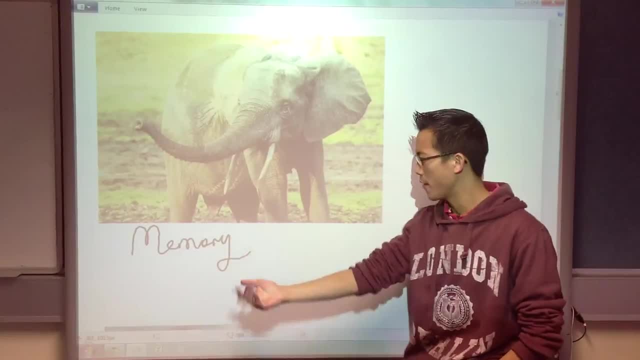 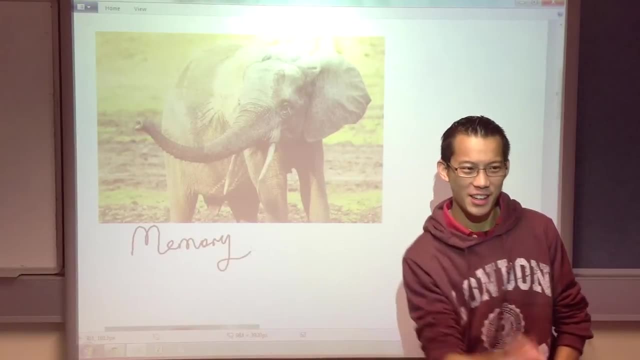 What advantages does? you can tell me this, right. Why does an expert system have a memory advantage over an expert? Because it's not human. Thank you for stating the definition of an expert system. Okay, so it's computer-based, so what? What does that have to do with memory? 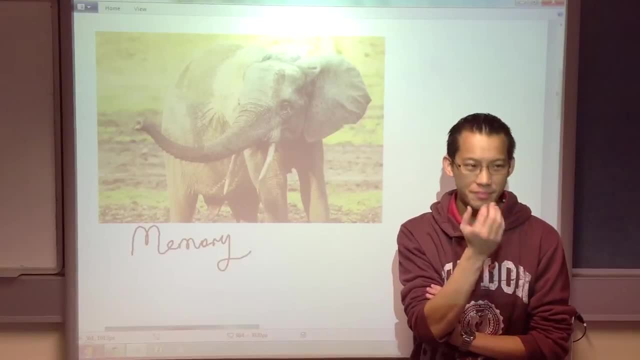 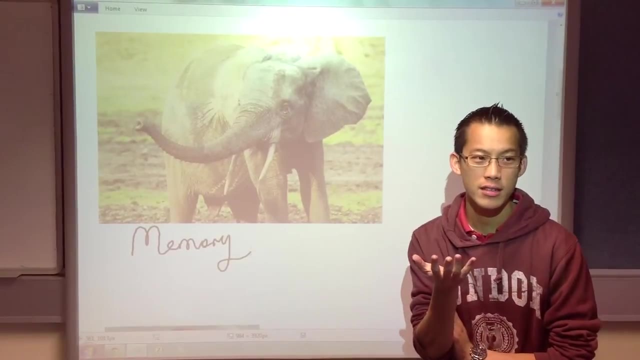 Yeah, Leo. Yeah, that's right. Like I mean, they say the working memory of a human being is five objects, five items plus or minus two. Okay, so if you're pretty good, you can get up to seven things. 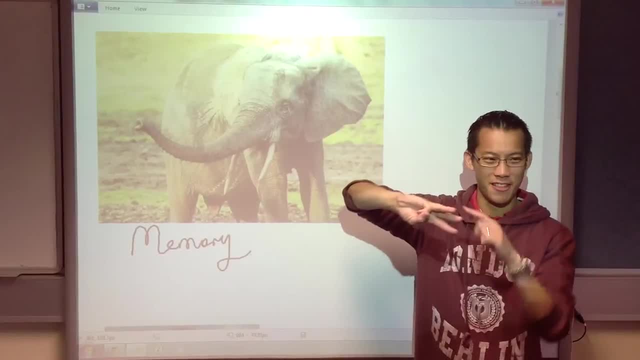 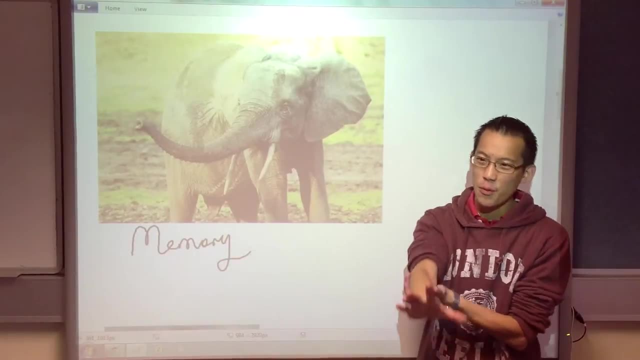 and if you're not so great, sort of do three things and end up with the fourth one and you're like, ah, I can't remember. okay, So that's the limitation of our short-term memory. Our long-term memory is the same. I don't know what your memory is like from say, 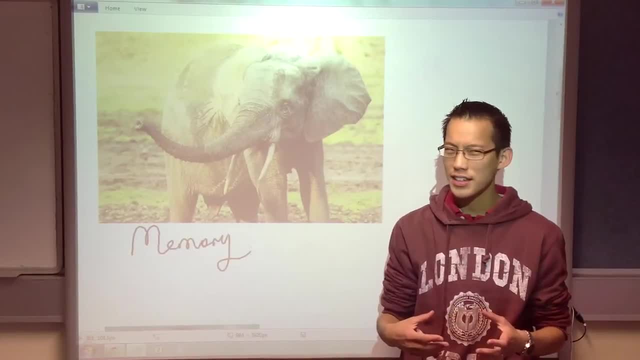 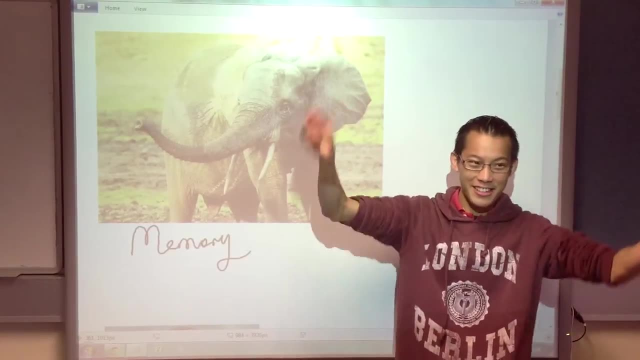 ten years ago, when you were like five, six years old. What kinds of things do you remember from back then? I only remember very, very few things, mostly the really traumatic things, right, And the things I really enjoyed. The rest of it is just. 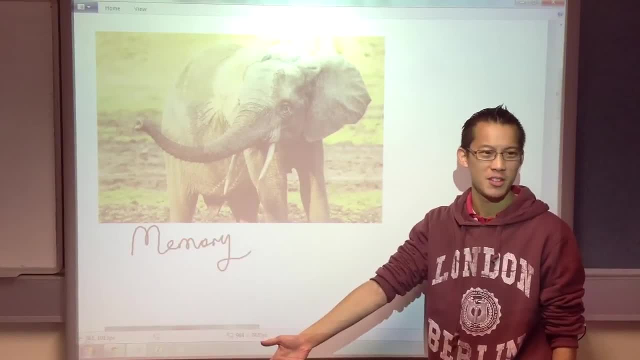 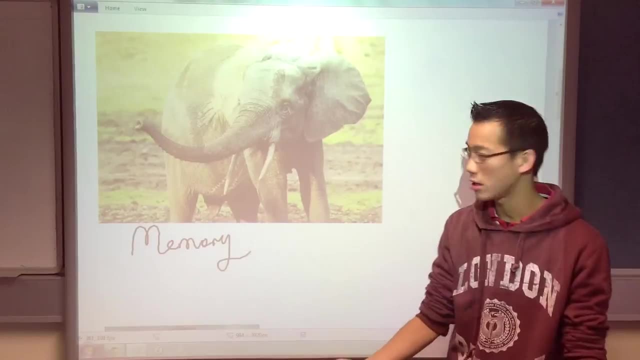 gone. okay, Which is quite astonishing, because you talk to a five or six-year-old like they know what's going on, Like they can speak language, they can read and so on, but we forget. Okay, so short-term and long-term memory computers have this. 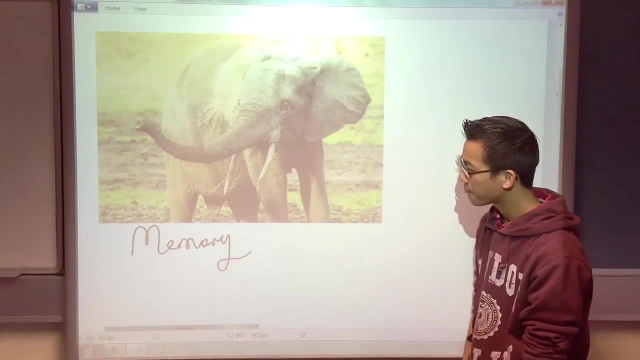 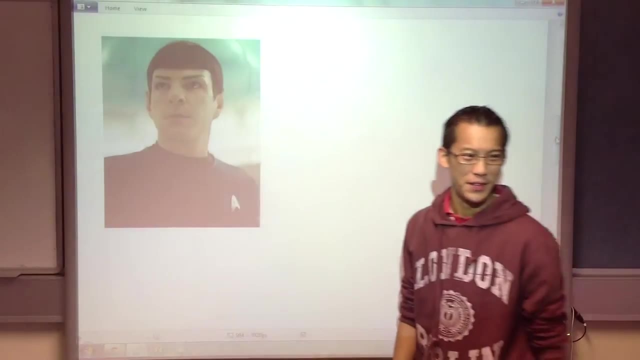 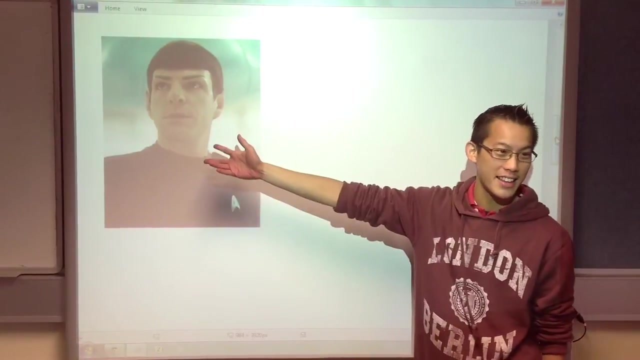 thing that they've got everything. it's all equally accessible to them, right? They never lose it due to memory loss. Okay, so there's a second advantage, Third advantage: The third advantage is Zachary Quinto. Now, what do you reckon He's dressed up as he's playing Spock in Star Trek. 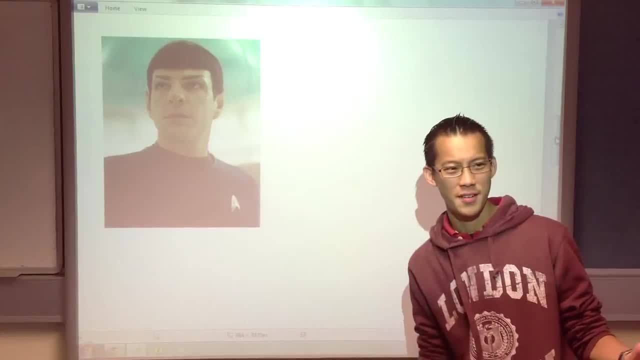 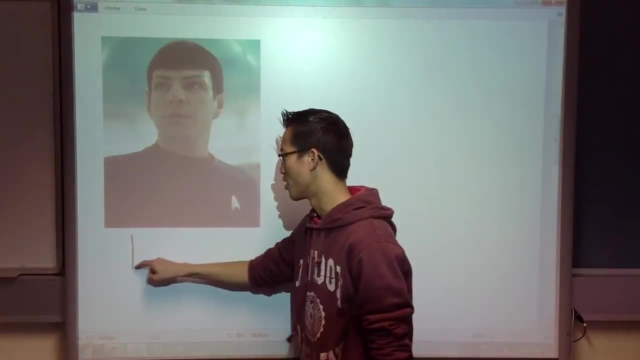 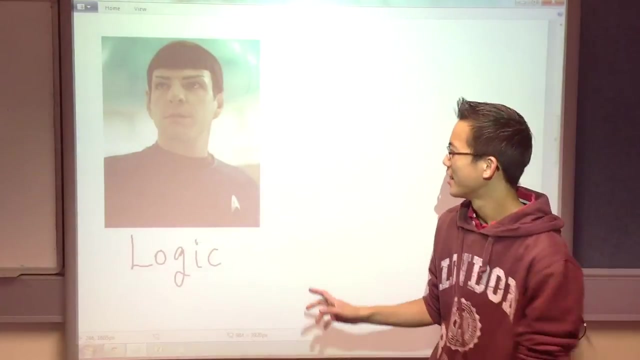 okay, And Spock is famous for- does anyone know, Live long and prosper my day. The thing is, his characteristic that he's most famous for is logic, alright, Logic. So if you've watched the movies or you know the stories, there's sort of a big contrast between Spock.